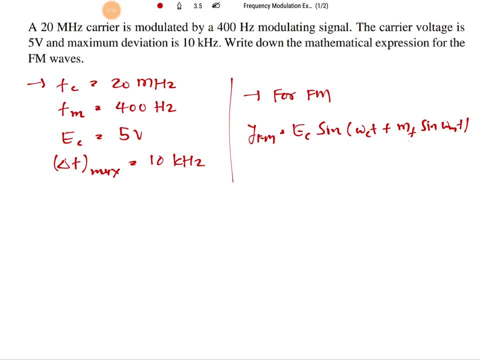 fm ec. but we need to calculate what is mf modulation index. So modulation index that we can calculate by mf is equals to delta f by fm, and that is 10 kilohertz. that is delta f and fm, that is 400 hertz, means 0.4 kilohertz. 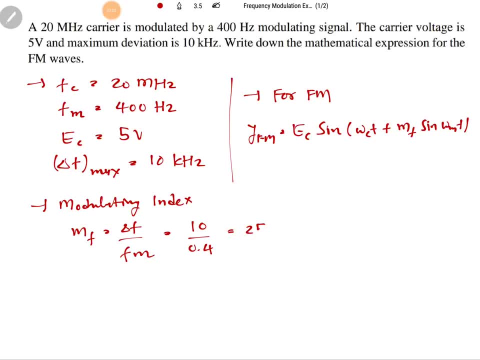 And if we calculate this you will be finding it is 25.. So now we can write fm signal, So fm signal, So that is ec. So that is given by 5 voltage into sin of omega means 2 pi f. So 2 pi into fc, that is 20 megahertz. 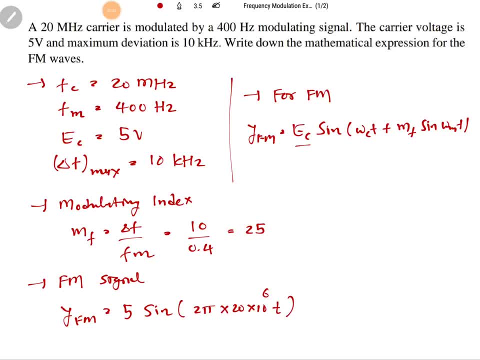 So 20 into 10 to the power, 60 plus mf, that is 25. that is this into sin of omega m, that is 2 pi into 400.. So that is 800 pi t. So this is what our fm signal in case of given data. 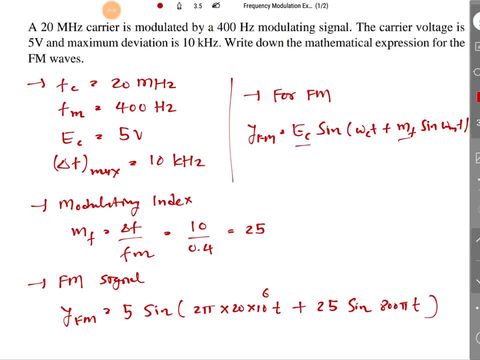 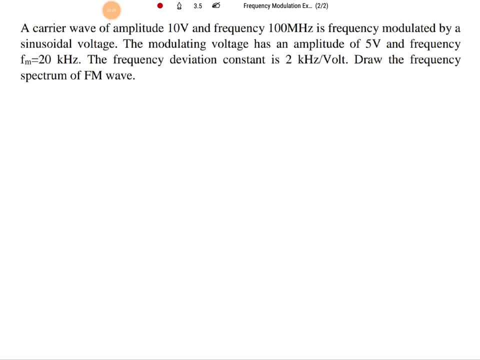 that is how we can solve this problem. now let us move on to next problem. now see in this problem a carrier wave of amplitude is 10 voltage, so let us write all those data. ec is equals to 10 voltage, frequency is 100 megahertz, so fm that is 100 megahertz. 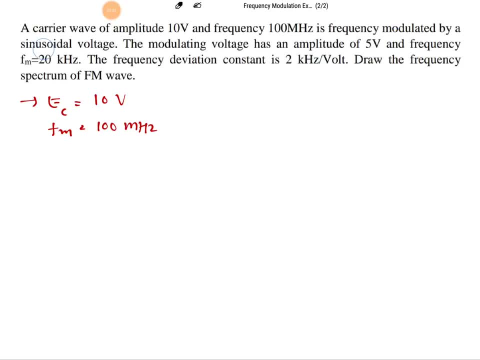 so frequency of carrier is 100 megahertz modulated by sinusoidal voltage. the modulating voltage has amplitude, 5 voltage. so em, that is 5 voltage, and frequency of that is fm, is equals to 20 kilohertz, frequency deviation constant, so that is 2 kilo hertz per. 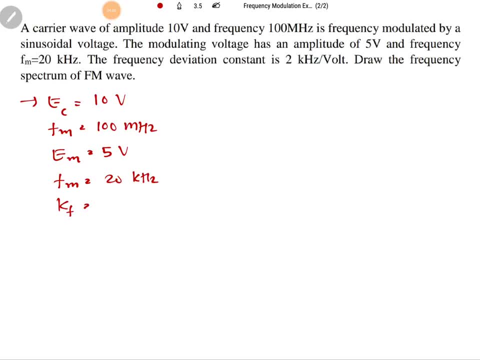 volt. so here frequency is sensitivity kf, that is given 2 kilohertz per volt. draw the frequency spectrum of fm. so we are delivered to draw frequency spectrum of fm. now see here, first of all we need to identify what is modulation index, and once we have modulation index we can calculate basal's coefficient. so 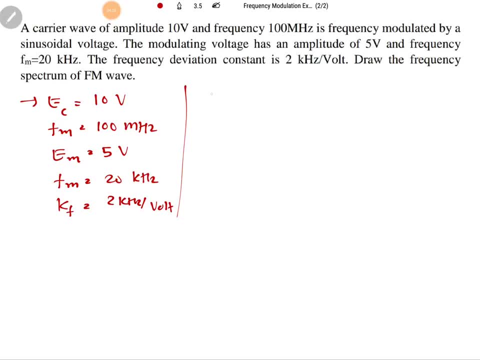 let us solve modulation index. so modulation index that is based on frequency deviation. so first we need to calculate frequency deviation. so frequency deviation is frequency sensitivity into em. frequency sensitivity is given 2 kilohertz per volt into em, that is 5 voltage. so maximum deviation that is 10 kilohertz. now modulation index mf. 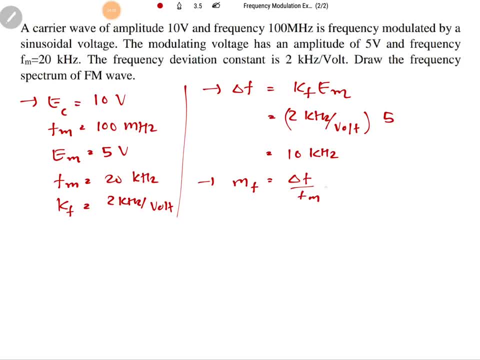 that is delta f. by fm. delta F is 10 kilohertz, FM, that is 20 kilohertz. so modulation index is 0.5. now we have this modulation index, so from that calculate basals parameter j1, j2 and j3 by table, so by using: 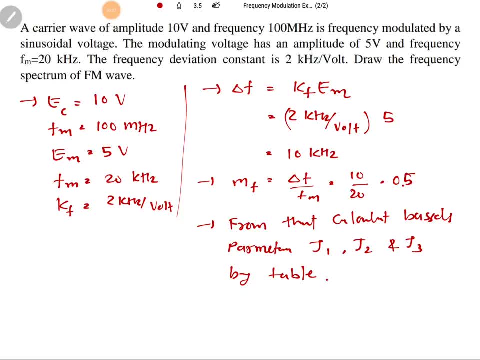 table one should calculate basals parameter. Now, I am not having that table right now, but you can see that in book. you will be given with this table and from that you will be having j1, j2, j3. so what I will be doing is 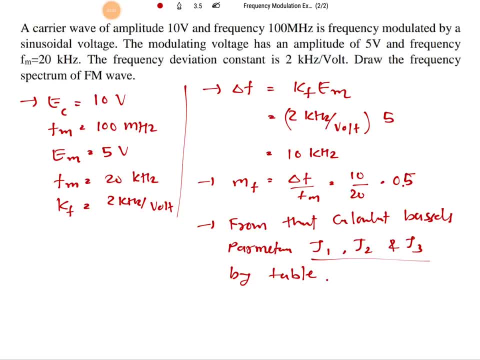 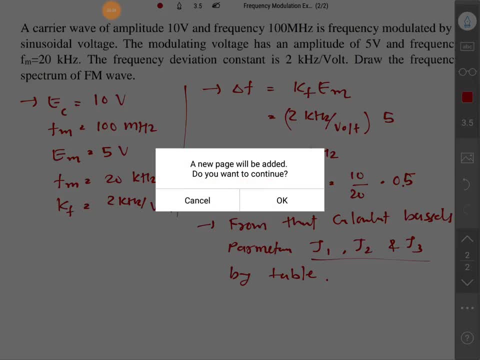 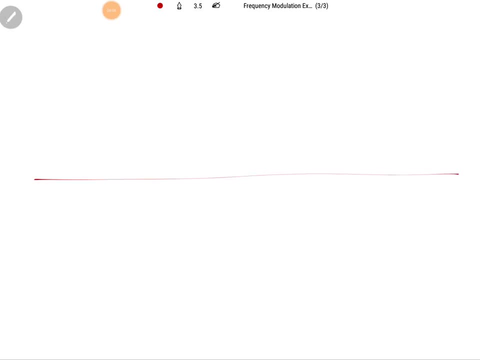 I will be writing all those things in terms of j1, j2, j3. so here question is to draw frequency spectrum of FM signal. Now, if you see frequency spectrum of FM signal, then in that frequency spectrum you will be finding. So At center there is carrier, and that carrier that we already know, that is fc, and here it. 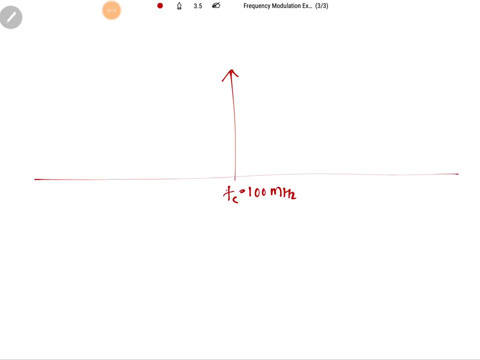 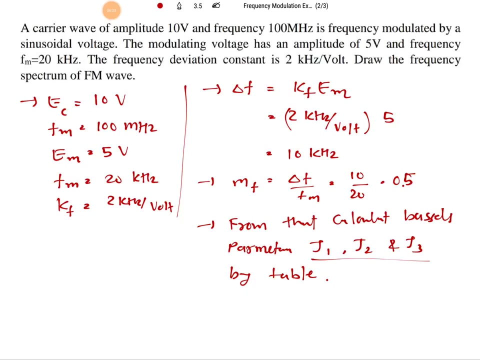 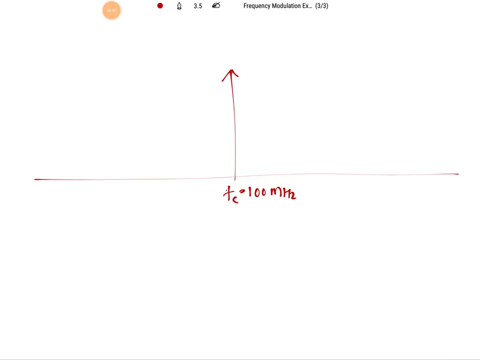 is 100 megahertz. Now if you see our previous calculation, then you will be finding here deviation. so that is what: 10 kilohertz and modulation frequency, that is 20 kilohertz. So here next band means first bands, so that will be having little lower magnitude with 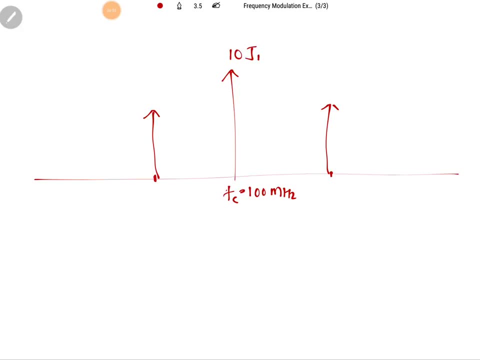 carrier magnitude is 10 j1. with first band magnitude is 10 j2, where 10 is amplitude of carrier signal. Second band That will be having magnitude that is 10 j3 and you will be finding it is decreasing. So obviously j2 is lower than j1, j3 is lower than j2. that is how it will decrease. and deviation: 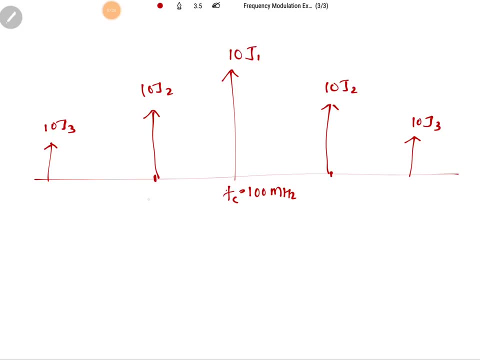 of frequency, that is what based on modulation, signal frequency. So here you will be finding that frequency should be fc minus 2 FM and here it should be fc fc plus 2 FM. So if you calculate that 100 megahertz minus 2, 20 minus 2 into that 10, so that will result. 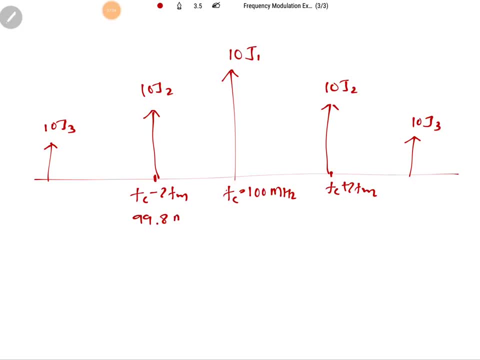 into 99.8 megahertz, third band that will be having frequency fc minus 3 FM over here. this will be fc plus 3 FM, So fc minus 3 FM, that will be 99.. Sorry, it will be fc. that will be fc minus 4 FM and fc plus 4 FM. 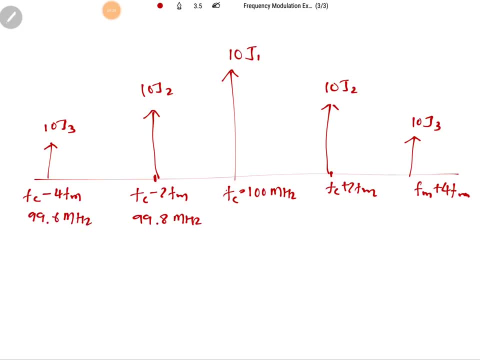 So this has to be 99.6 megahertz And over here it will be This, much right. So hundred point four megahertz and F C plus 2 FM. that has to be hundred point two megahertz. and here this F, j1, j2, j3, so that we can identify based on bezels.